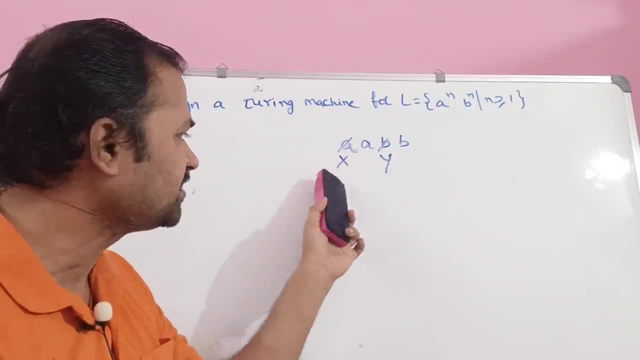 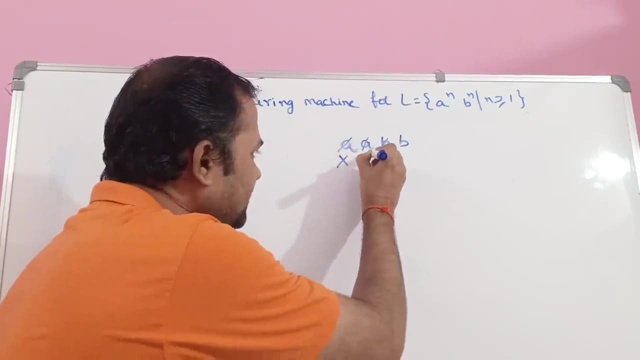 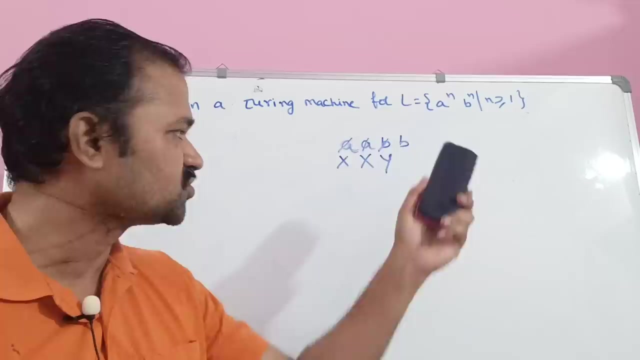 x. So here we have x. So after that we have to move the. we have to move the read rate head towards the right, So here we have a. So replace this a With x. Next, we have to move the read rate head towards the right till we get b. So here we have. 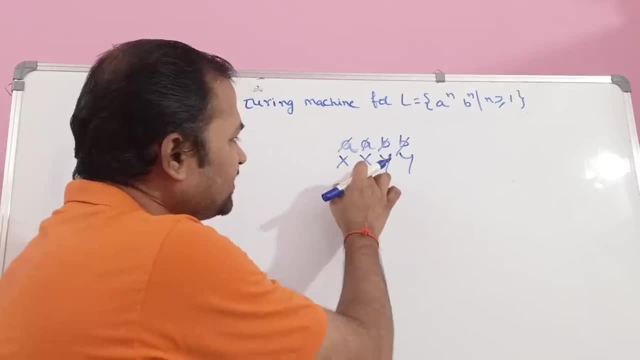 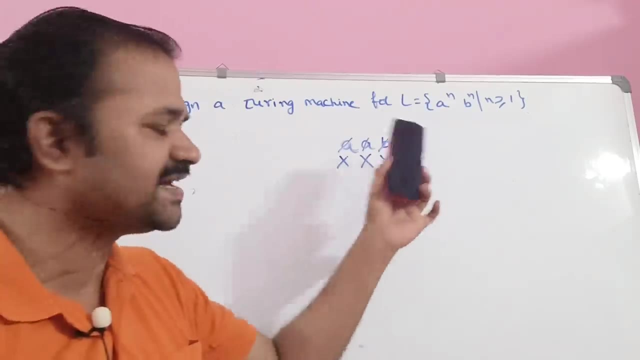 b. So replace this b with y. So for this a we have the corresponding b. So here we are replacing this b with y. So this is an example. Here we have 2 a's and 2 b's. The 2 a's are replaced. 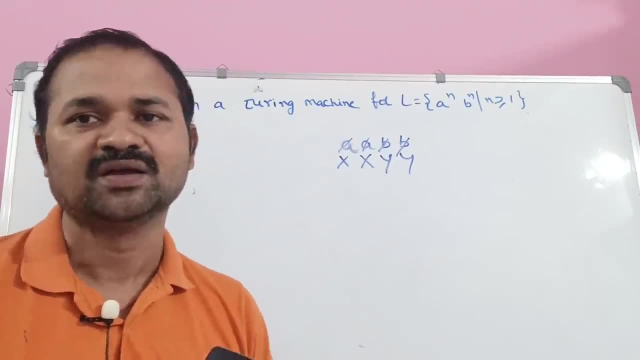 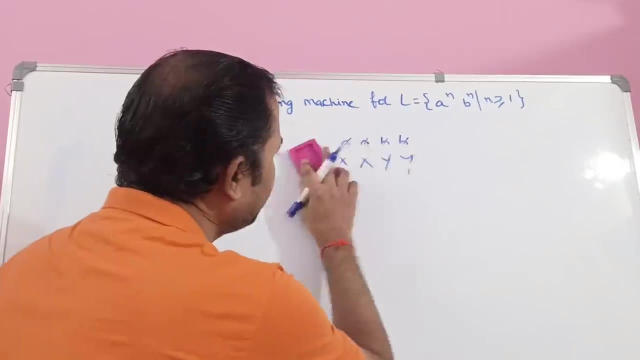 with 2 x's, and the 2 b's are replaced with the 2 y. Now, with the help of an example, let us design the Turing machine for this problem. So let the string is 3 bull, a, 3 bull, b, 3 bull. 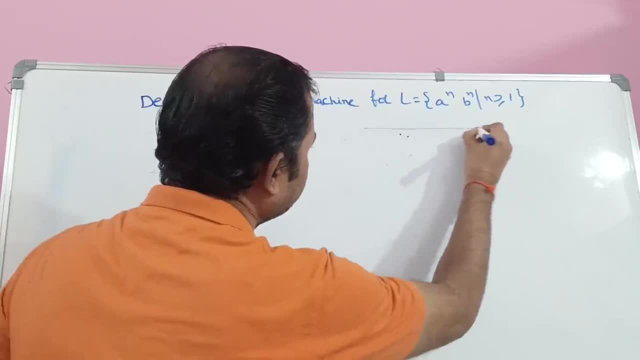 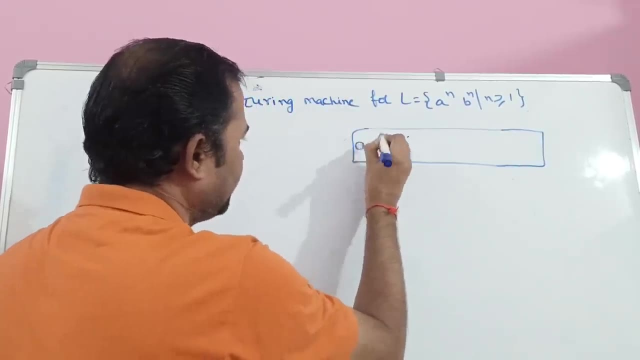 a, 3 bull b. So let, this is our string. So let us take 3 bull a, 3 bull b, So that all the cases will be taken. So let the string is 3 bull a, 3 bull b. So let us take some bigger. 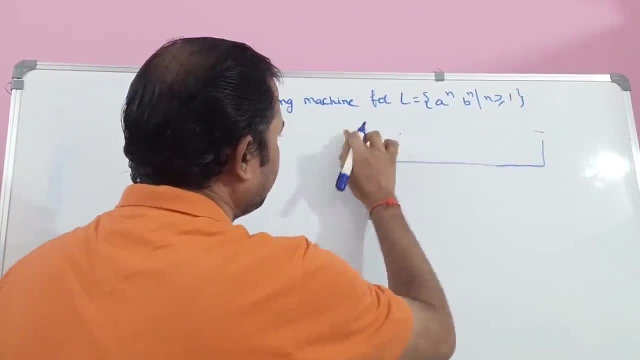 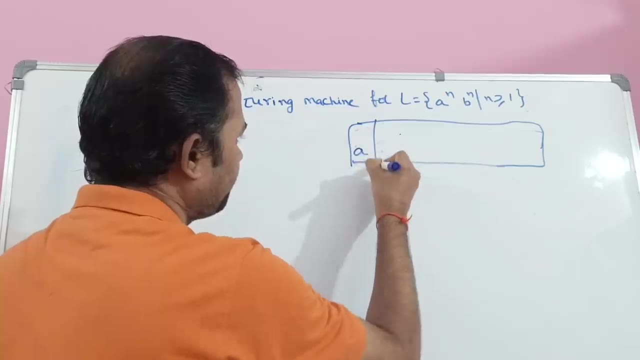 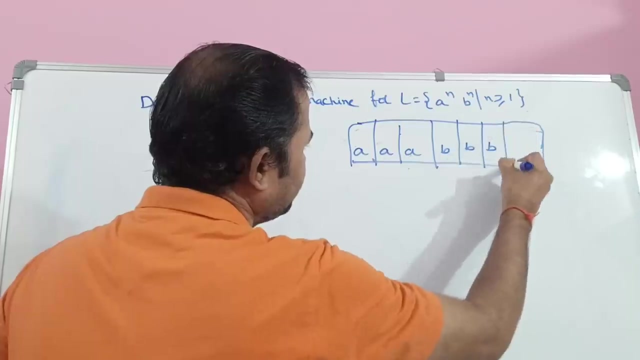 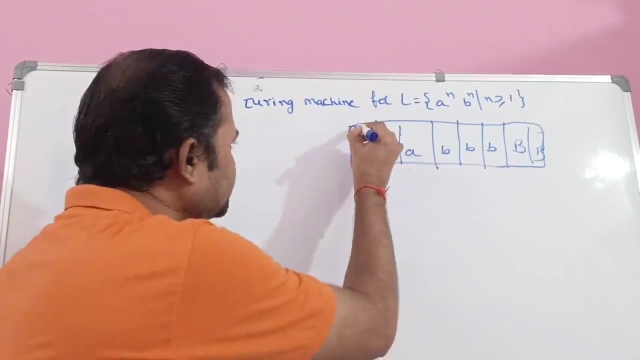 diagram. So let the string is 3 bull a, 3 bull b. So a a, a, b, b, b. So after this we can have n number of blank spaces. We can take n number of blank symbols. So here, also before this, we can have n number. 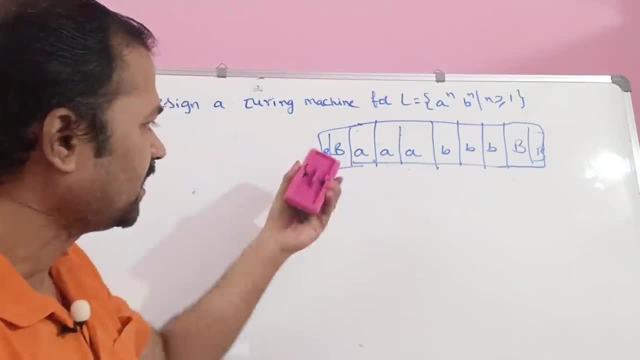 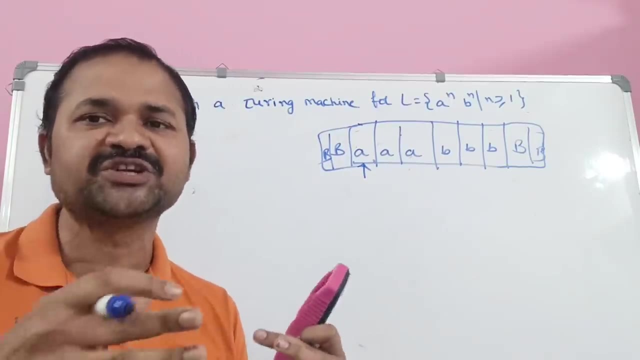 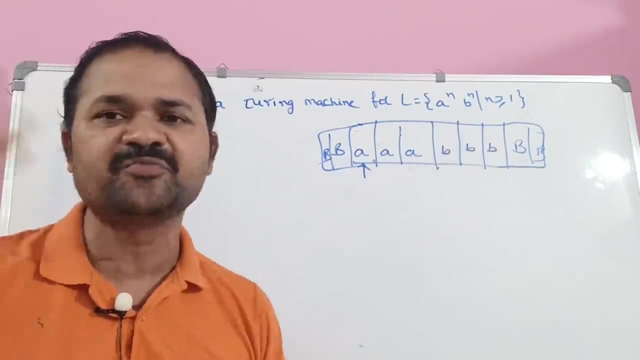 of blank symbols. Ok, Here, this is the read rate head. We know the advantage of read rate head: Perform both read operation as well as write operation. So write operation means change the content of a to some other content, Change the content of b to some other content, As 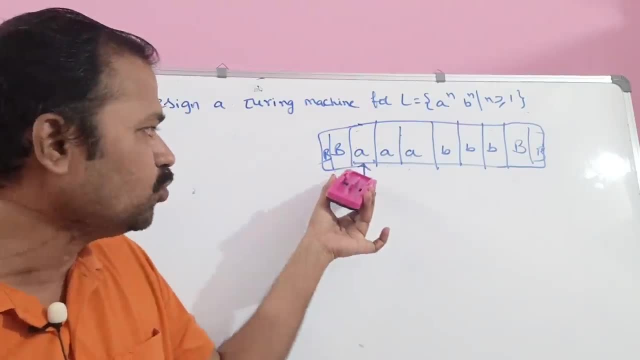 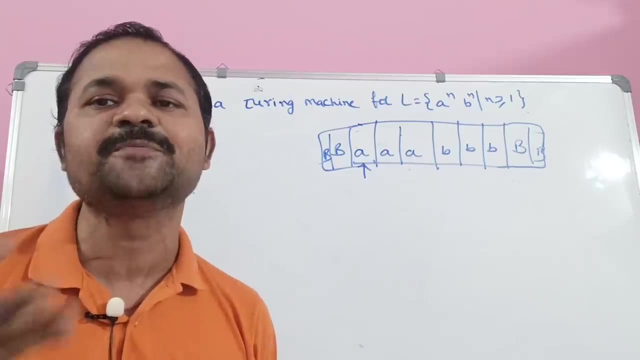 well as one more advantage of the read rate head is we can move either from left to to right or from right to left, Whereas that provision is not available in the finite auto, meta and PDA. In finite auto and PDA, we can move only from left to to right, Whereas here. 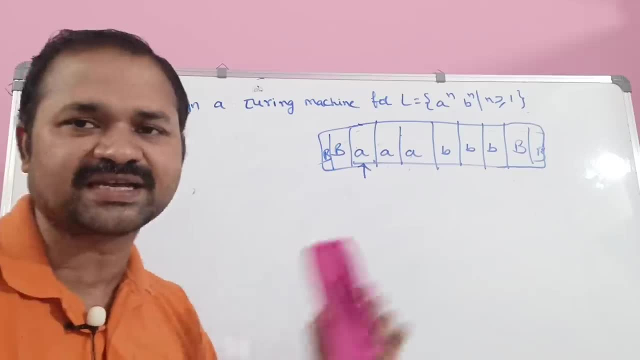 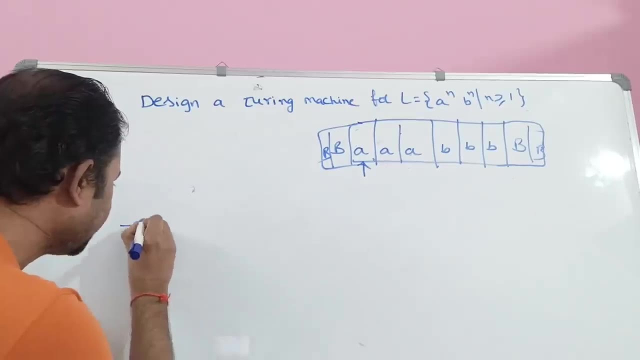 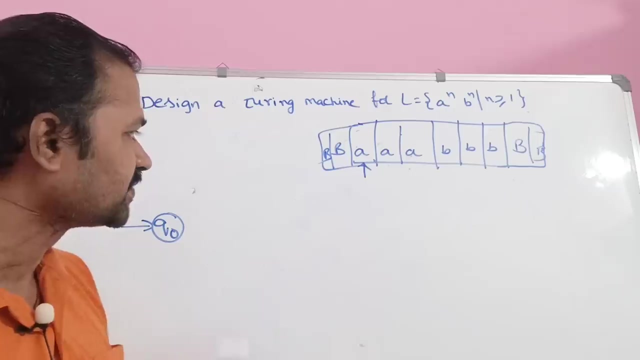 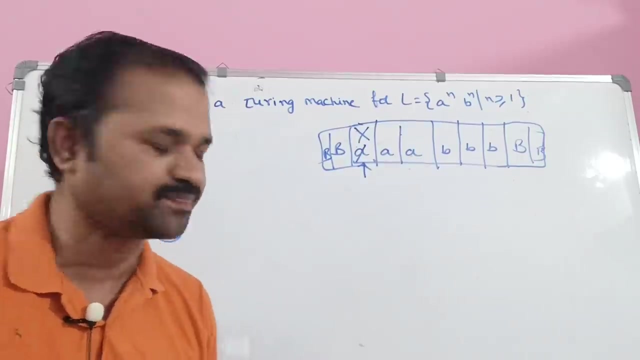 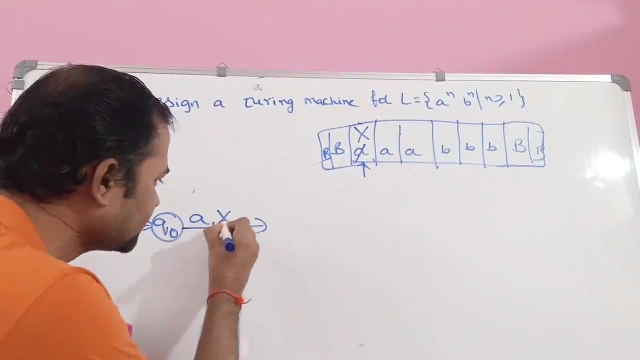 we can move in both the directions. So we can then construct the diagram here, Transition diagram. So let the starting state is q naught, If we read a, then change the content of the a to x and move the read rate head towards the right. So if we read a, then change the content of a to x and move the. 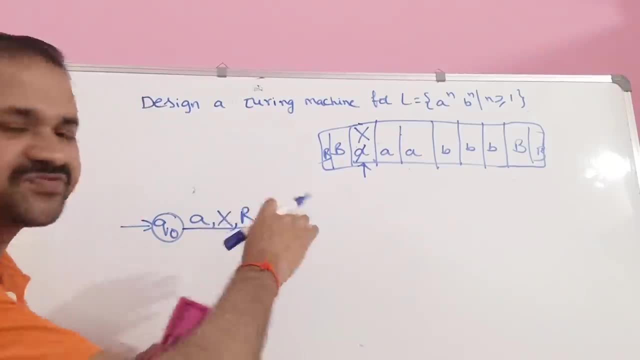 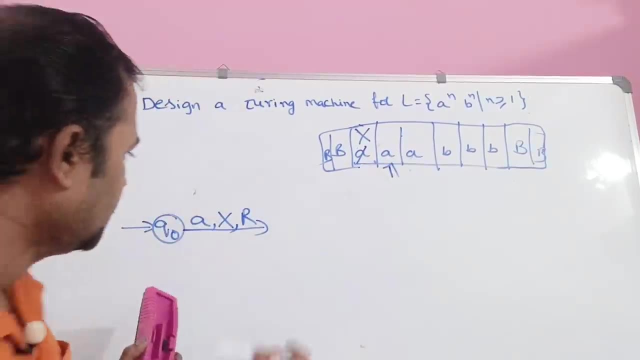 read rate head towards the left. So now here, first, we are going to understand that A Chinese head towards the right, so r stands for we are moving towards the right. okay, so now the read rate head is at this location. let let the next state is q1. so if we read any number of yes, then 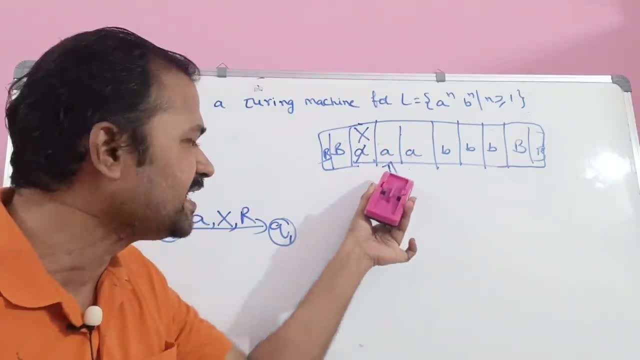 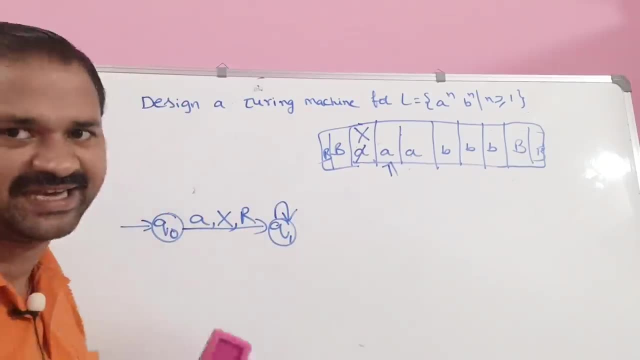 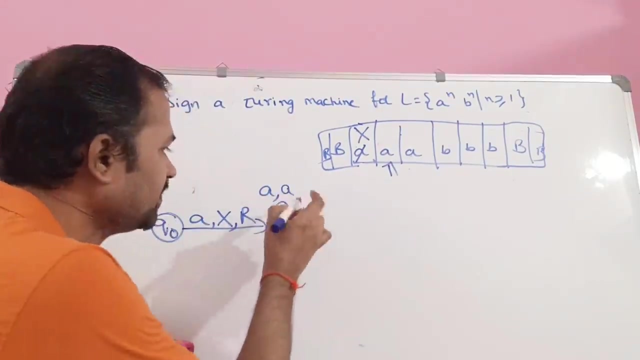 there is no need to change them. we have to simply move the read write head towards the right till we get b. okay, so here there is no need to change any state here. so if you read a, then there is no need to change a, so write a only and move the read rate here towards the right. so here we have a. there is. 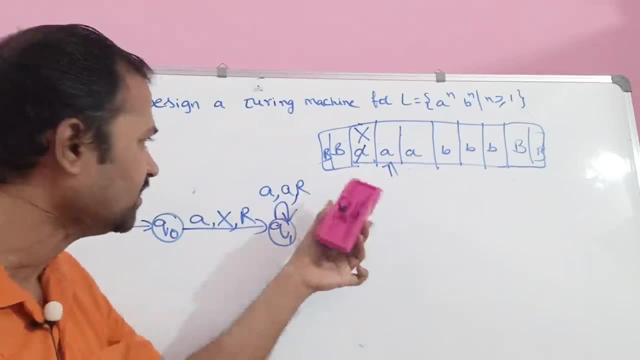 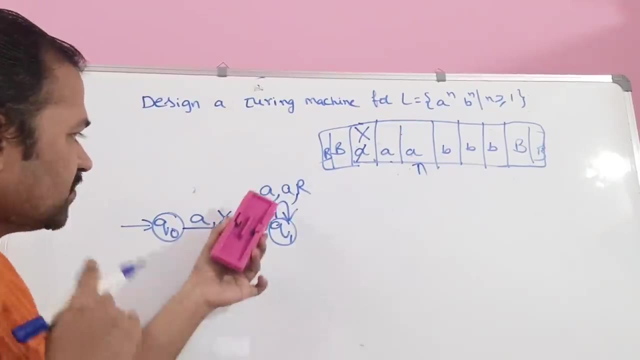 no need to change the a. so that's why here we have written a very and move the read rate head towards the right. so now the read write head is at this location. so here we have a. so replace with a only so if a won't change. 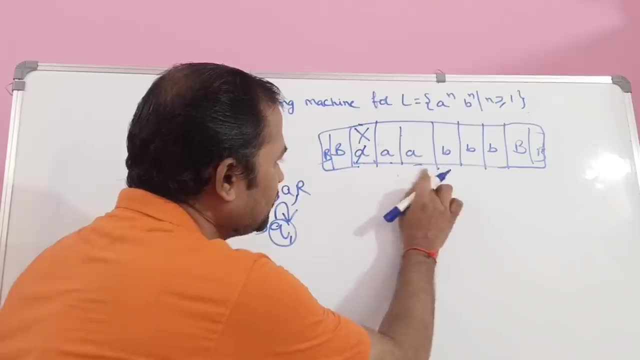 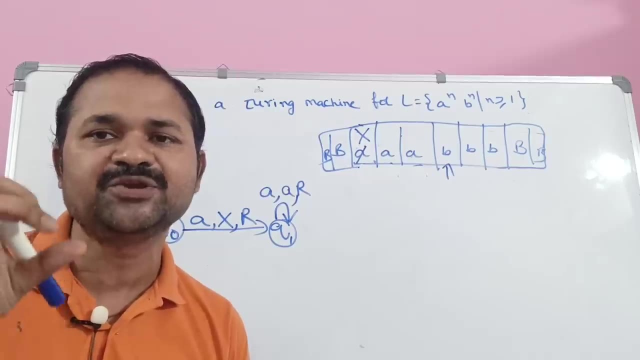 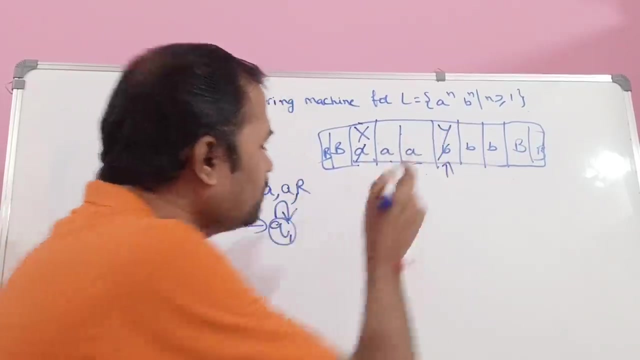 changes and move the read write head towards the right. so now the read write head is at this location, okay. so next, if we read b, then change the content of the b to y, change the content of the b to y and move the read write head towards the left till we get the x. okay, so now we have to. 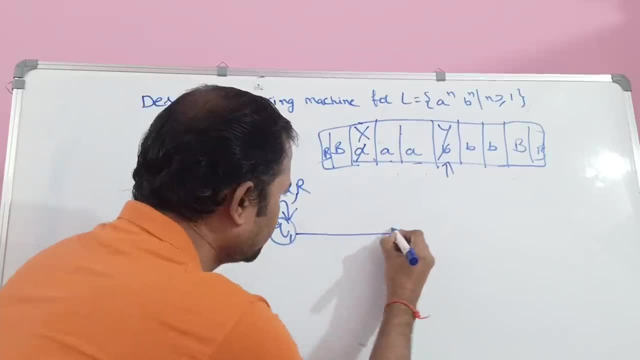 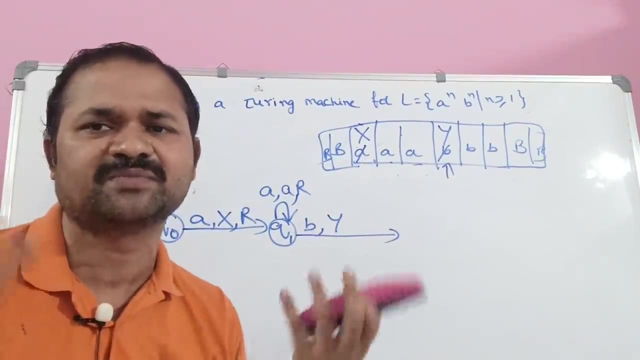 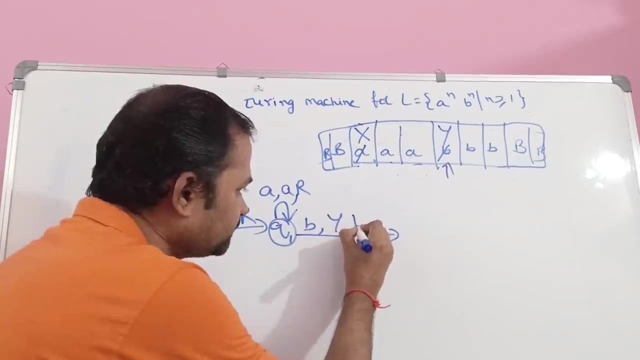 change the state from q1 to q2. so if we read b, then replace it with y. it is our choice. we can use some other variable also. we can use some other name also, there is no problem. and move the read. write head towards the left till we get x. till we get x. okay. so let us change from q1 to q2 state. 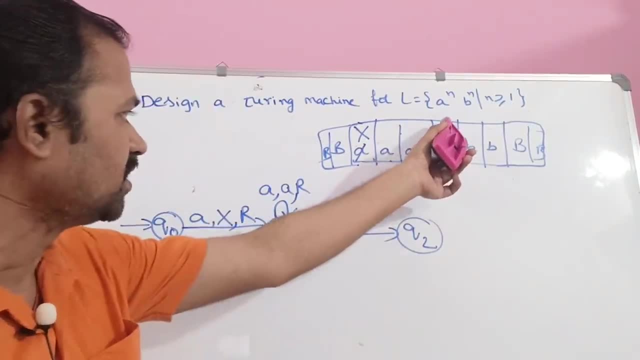 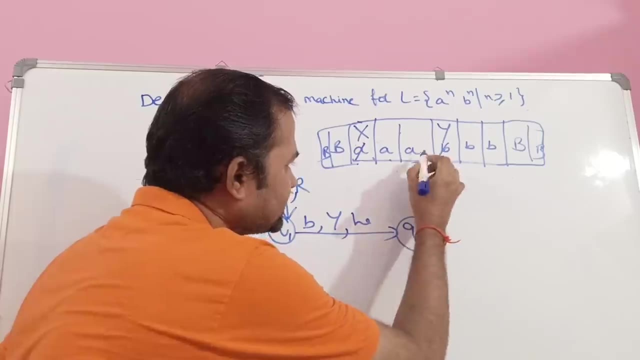 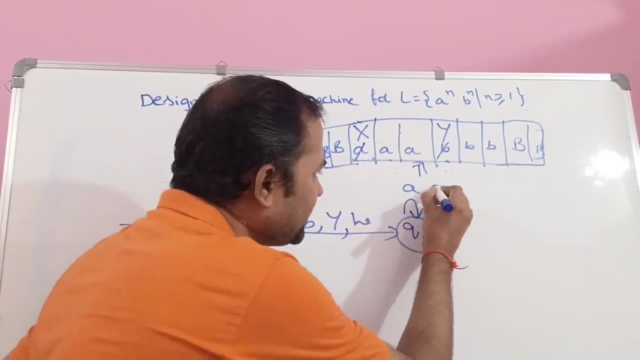 now, okay, so change b from, change b to y and move towards the left. now read write head is at this location. so if we read a, then there is no need to change the a. so keep a as it is and move the read write head towards the left. so here we. 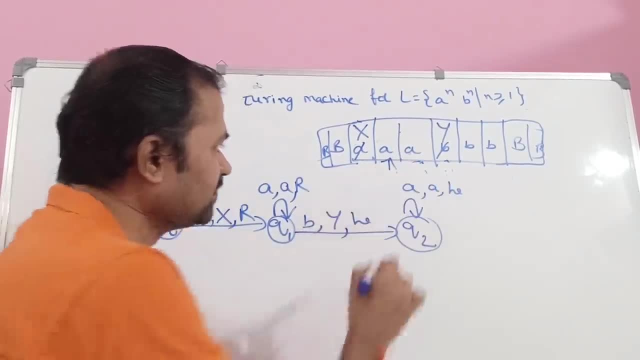 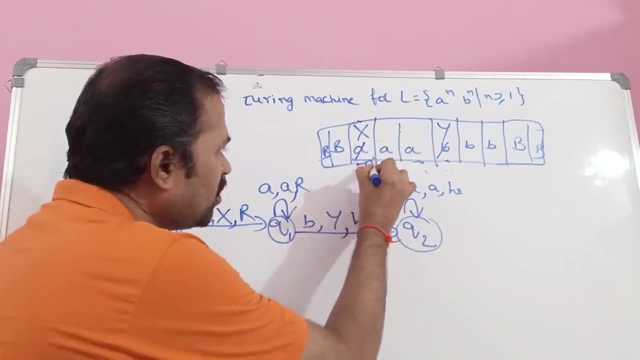 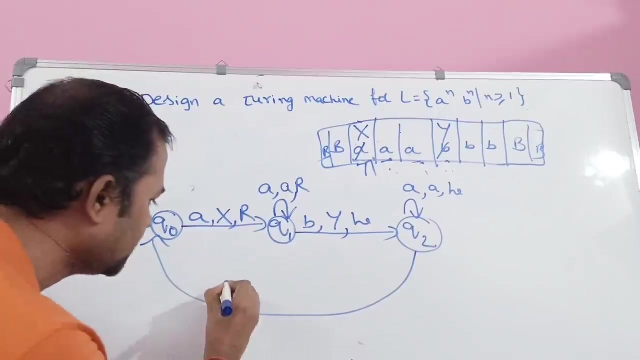 have a. no need to change a, so move towards the left. so again we have a, so no need to change. and move the read write head towards the left. so now, here we have x, so whenever we read x here, then write a transition like this: whenever we read x, then there is no need to change x, so right as x only. 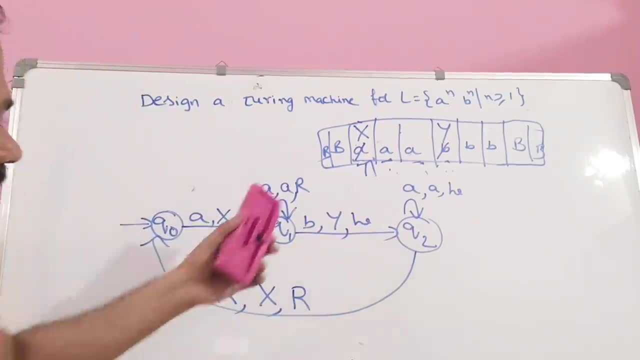 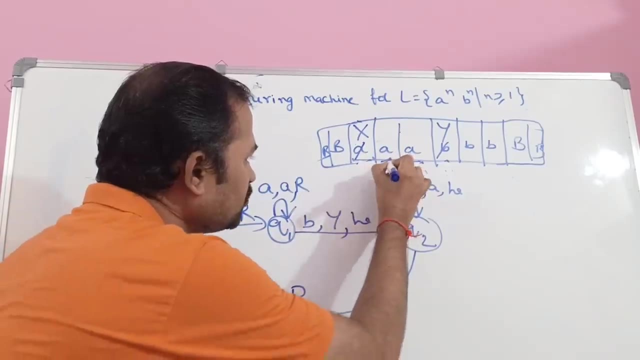 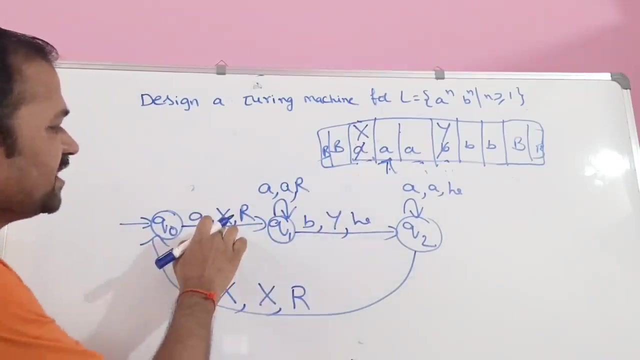 but move the read write head towards the right. okay, so here we have x. there is no need to change x, but move the read write head towards the right. so now the read write head is at this position. so again, a is applied on q. naught, if a is applied, then we have to replace a with x. so let us replace. 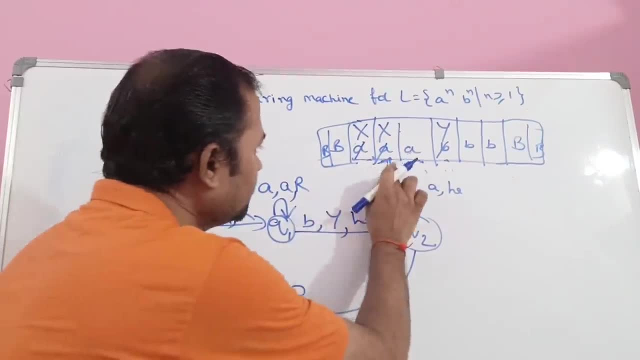 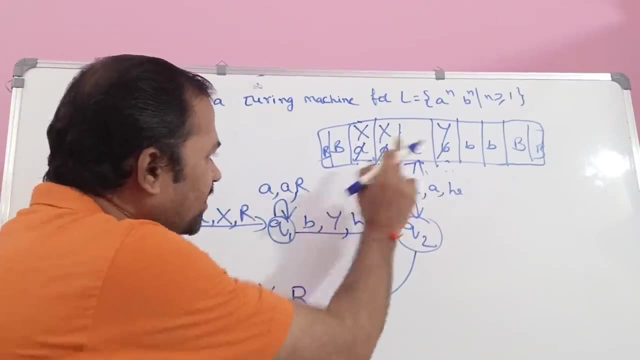 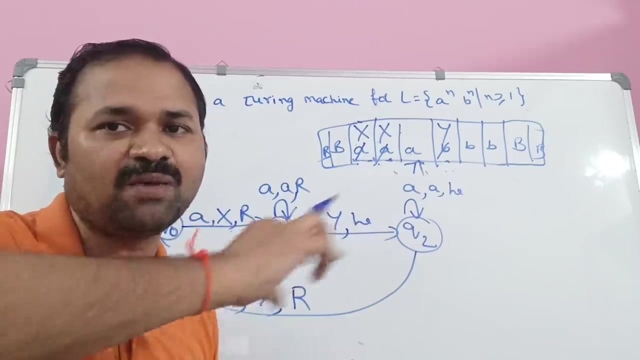 a with x and move towards the right. okay, so move towards the right. so now we are at q1 state. now we are at q1 state. so if we apply a on q1, then there is no need to change this a. why? because a is modified to x. now we have to move until we get the b. okay, so there is no need to change here. 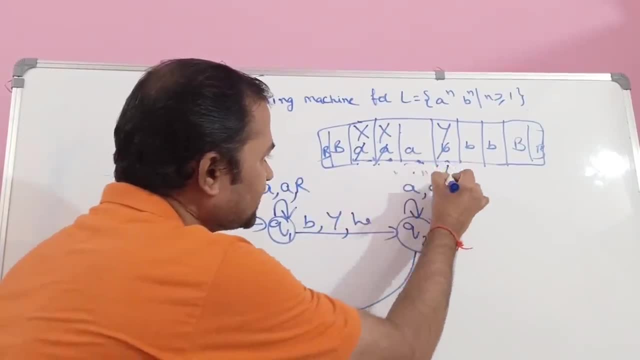 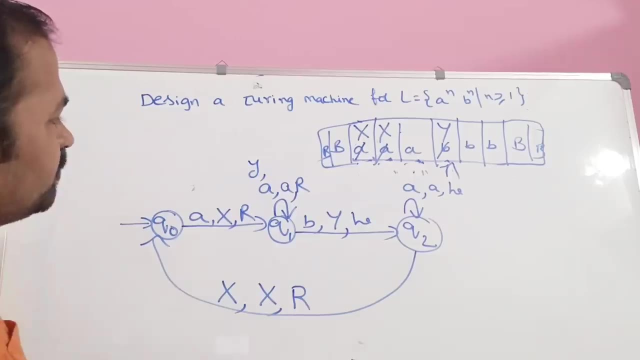 but we need to move towards the right, so move towards the right. next, here we have y. okay, so let us one more transition. so if we read y on q1, then there is no need to change y. there is no need to change y, but we have to move, read, write, head towards the right. there is no need to change the. 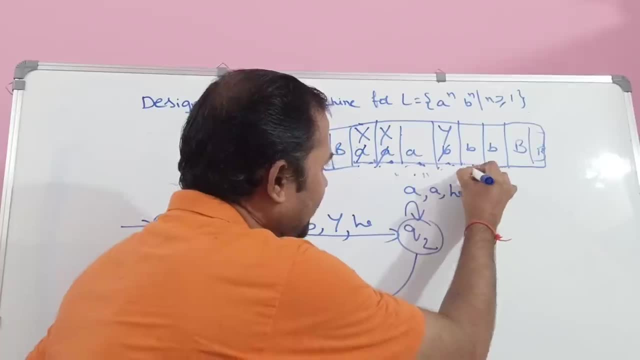 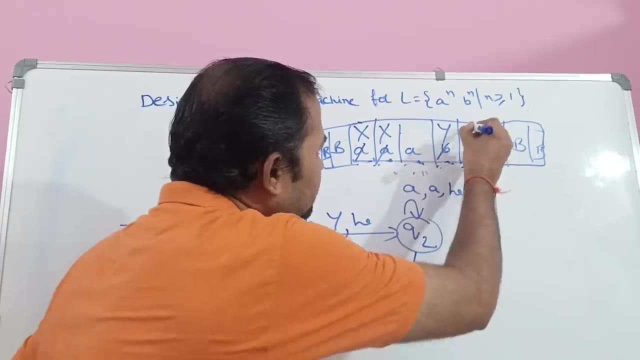 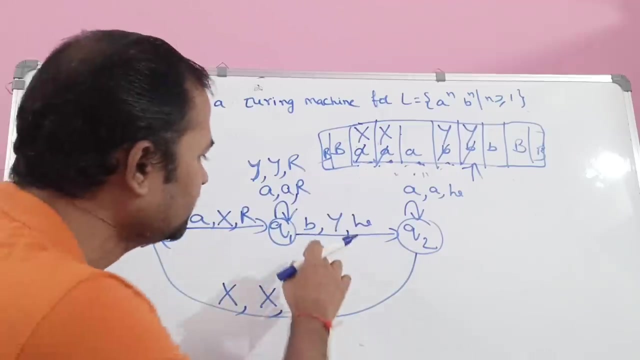 state here: so move, read write head towards the right. okay, so next here we have b. so if we move b, then replace this b with y and move the read write head towards the left and move the read write head towards the left. so now we have to change from q1 to q2, so mu q1 to q2. so now we 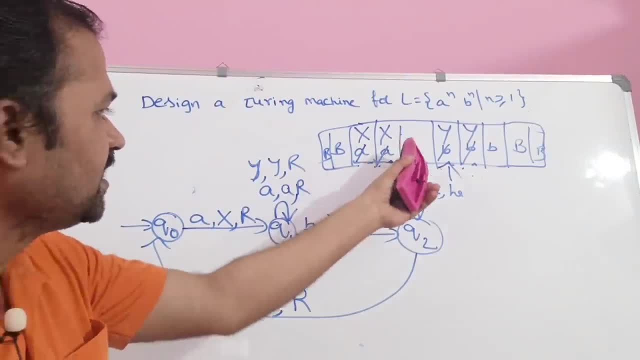 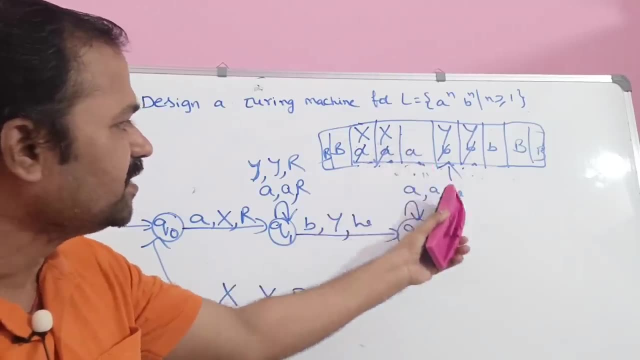 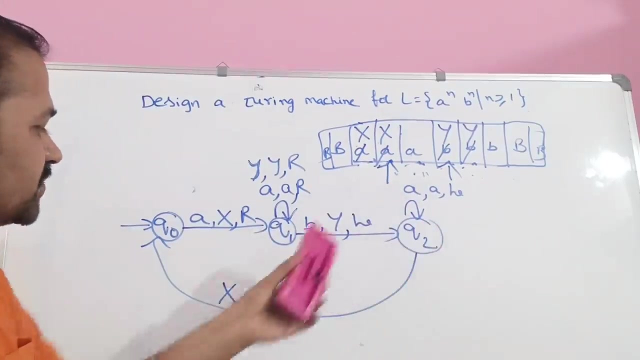 are at which state. q2 state. okay, here we have a. so if we have, if we apply a on q2, then there is no need to change a here and move towards the left. so now read write head is at this location. okay, if we read x on q2, then there is no need to change x. we have to simply maintain. 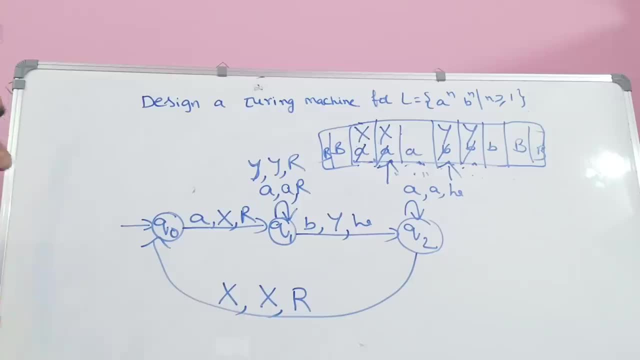 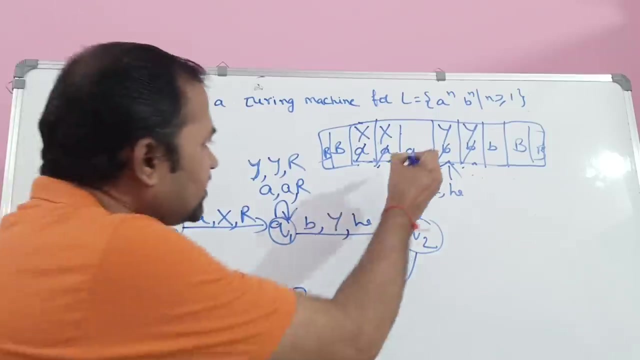 as x only, but move the read write heads towards the right. okay, so here we have x. there is no need to change this x, but move the read write head towards the right. so now we are at q0- q0. so here we have a. so if we have a on q0, then change the content to x. change the content. 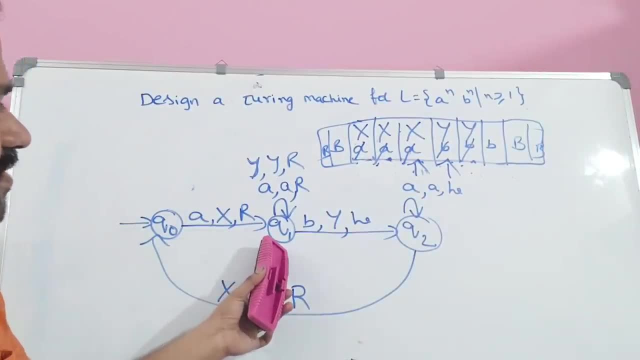 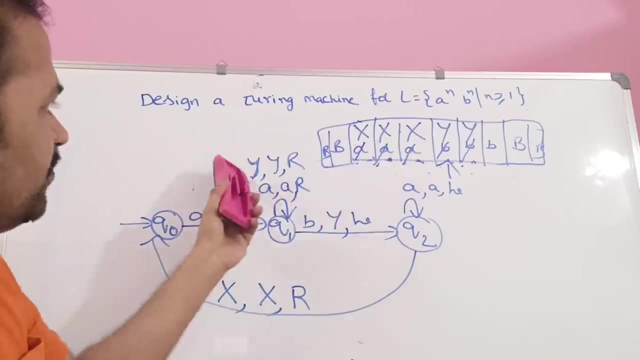 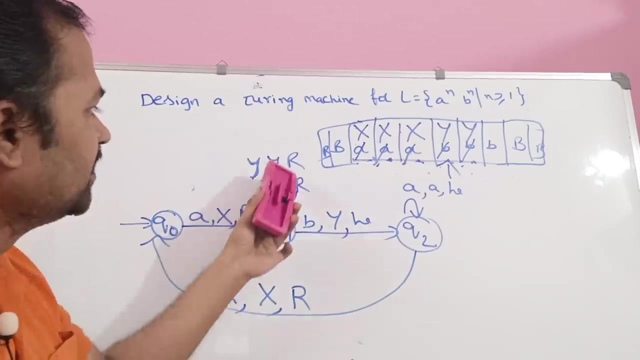 to x and move the read write head towards the right, and here that content is changed. here now it is a function of this location. so we applied y here. there is no need to change y. there is no need to change y. so that's why we have written y only. but we have to move the read write head towards. 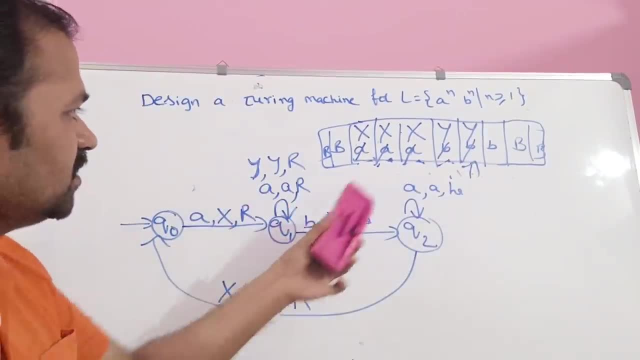 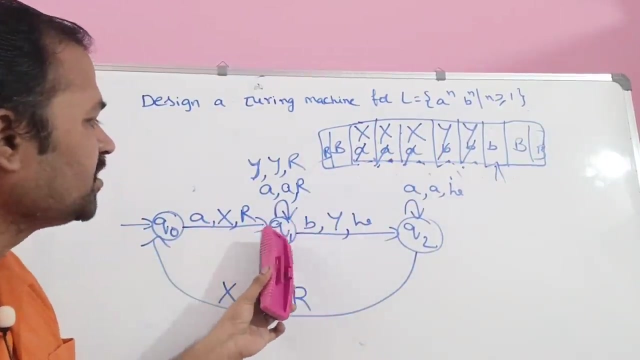 the right. so he, we are at q1. only, this is self loop. so again, uh, y is applied on the q1, so there is no need to change y, but we have to move, read, write, head towards the right. if we apply b on q1, then it should be modified to y. it should be modified to y, but we have to. 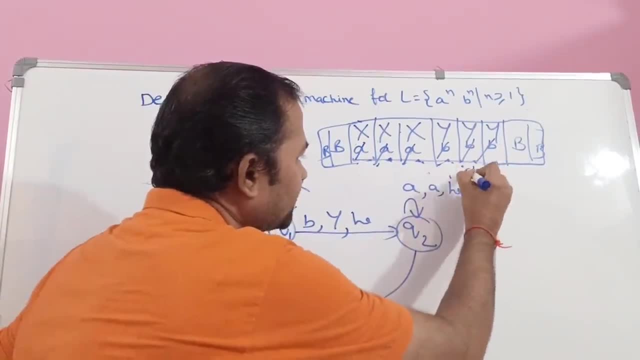 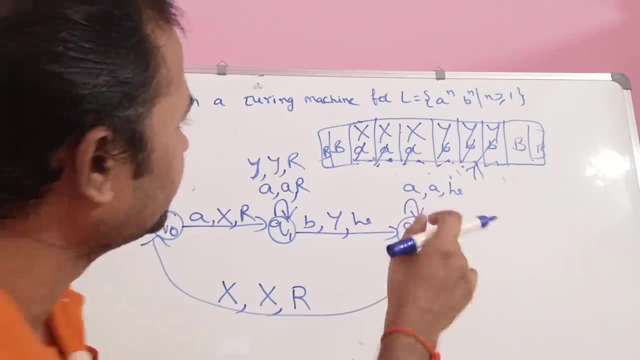 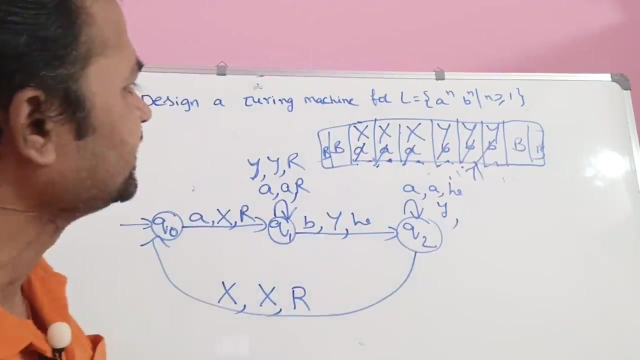 move towards the left, we have to move towards the left. so now we are at q2 state. so, on q2 state, on q2 state, if we apply y here we have y. ok. on q2 state, if we apply y, then there is no need to. 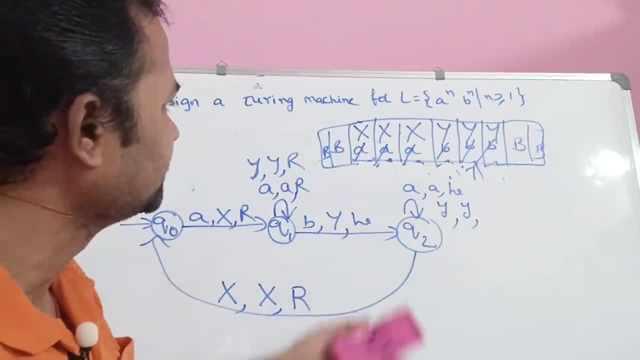 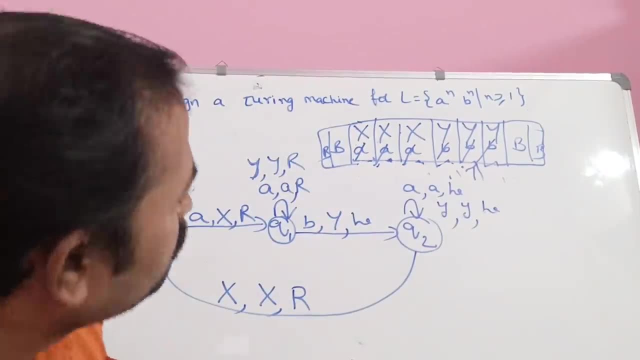 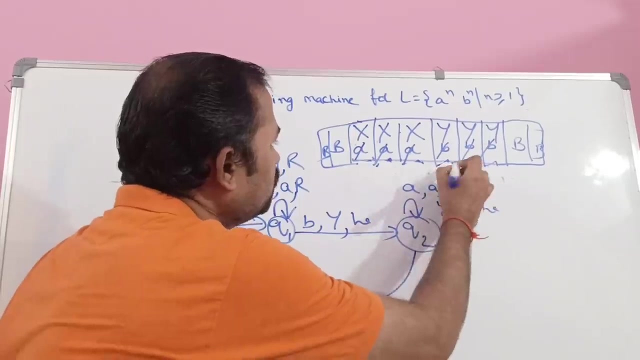 change y, so y. so keep y as it is, but we have to main move the read write head towards the left. we have to move the read write head towards the left. ok, so y, there is no need to change y, but we need to move read write head towards the left. so now the read write head is at this: 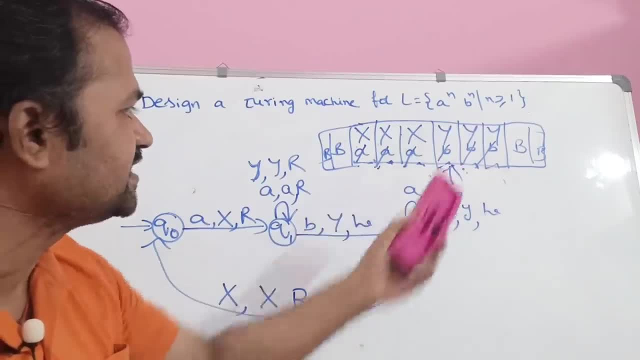 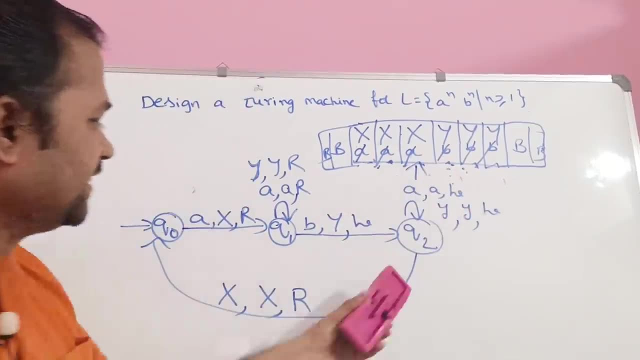 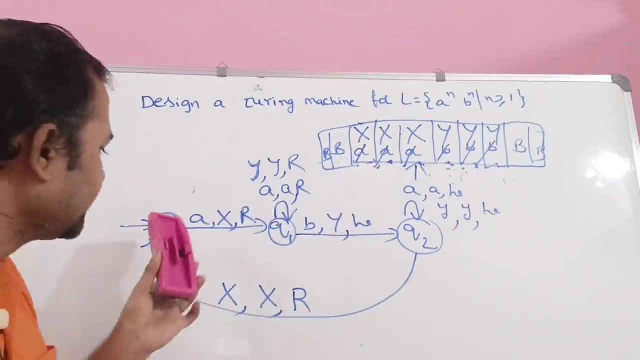 location only. so again y is applied. again y is applied, so there is no need to change y. but we have to move read write head towards the left. so next, x is applied. x is applied, so there is no need to change this x, but we have to move the read write head towards the right. so now we are at q0 state. 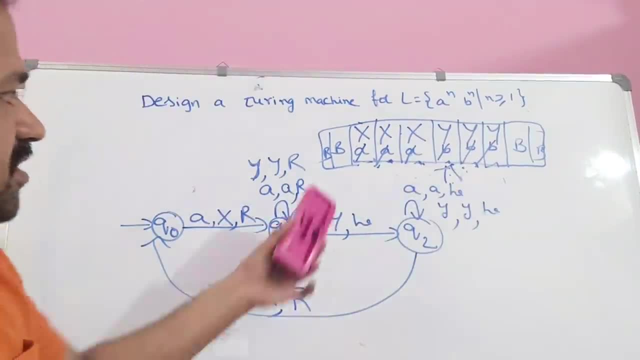 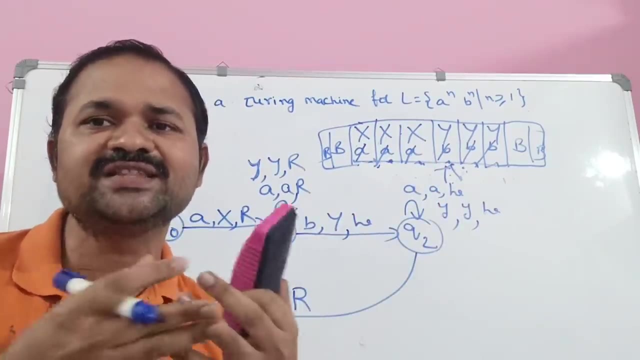 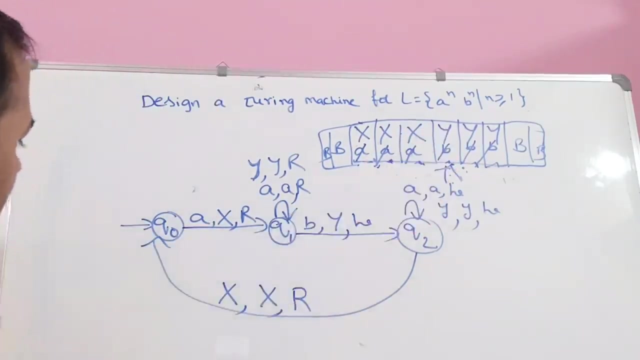 now we are at q0 state, so all the x's are completely readed. so after this x we don't have any other a, so we can say that all the a's are completed. ok, so let us check whether is there are any b's or not. so that's why, here on q0, on q0. 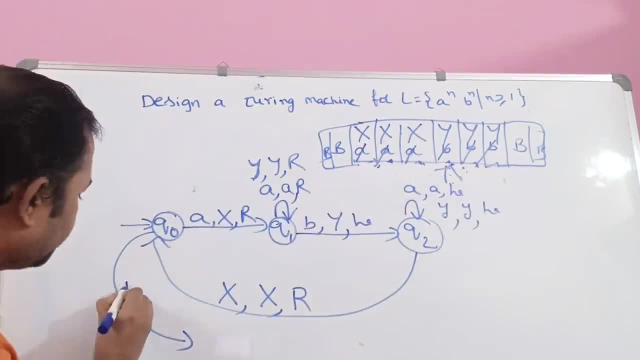 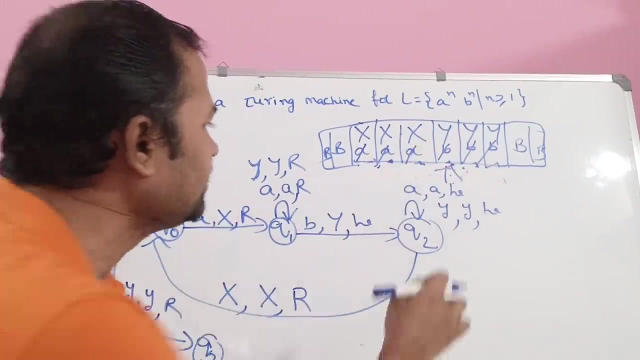 on q0: if we apply y, then there is no need to change y, but we have to move the read write head towards the right. so next state is q3, next state is q3. so on q0, y is applied, there is no need to change y, but we have to move towards the right. we have to move towards 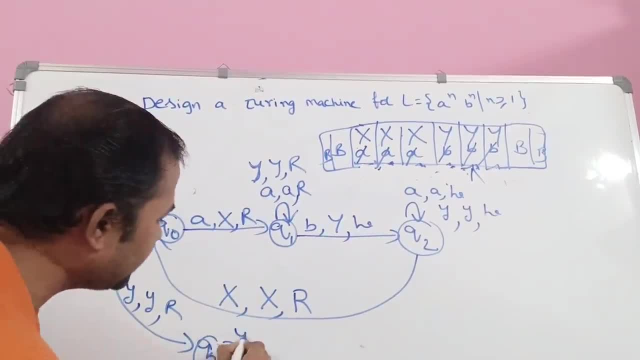 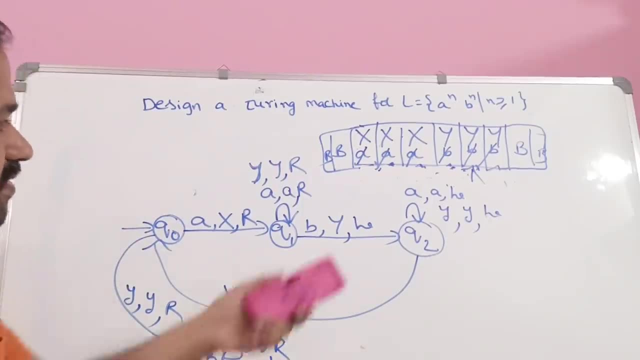 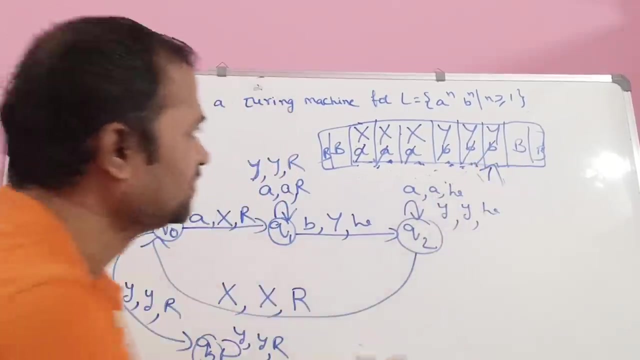 the right. so on q3, if we apply any number of y's, then keep y's as it is, but move the read write head towards the right. so here we have one more y. so keep y as it is, but move the read write head towards the right. so one more y is applied, so no need to change. 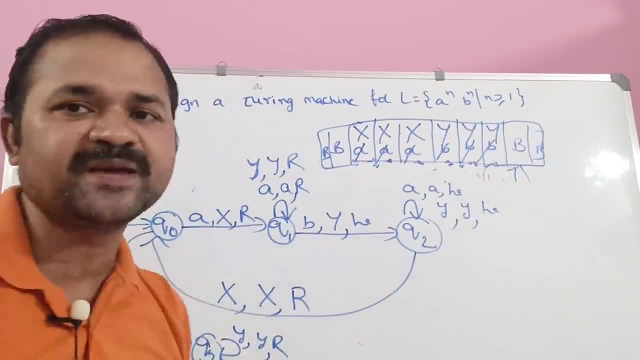 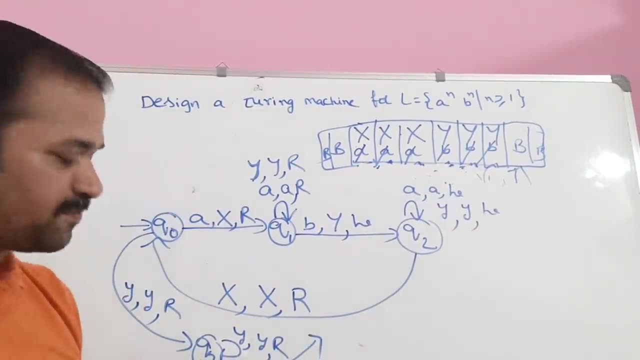 y, but move the read write head towards the b. so b specifies that blank symbol. so there are no other b's. ok, so that's why here whenever the blank symbol is applied. so here the transition is like this: so whenever, whenever blank sign is applied, then that is the reading write. 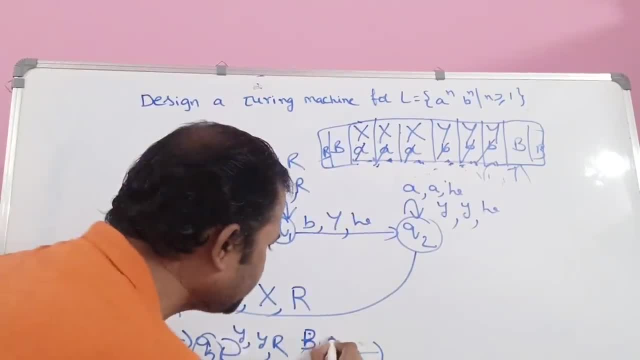 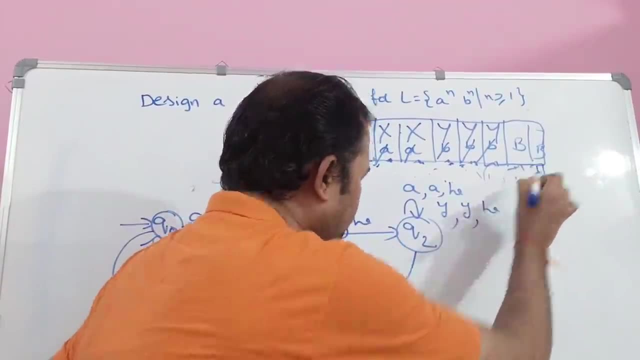 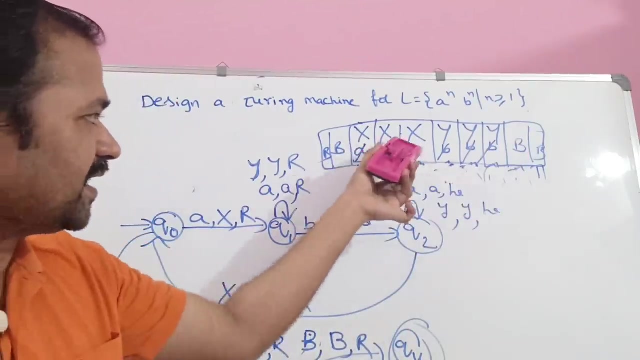 blank symbol is applied, then it should be replaced with blank symbol only. So let us move to the right. let us move to the right. So now we have moved to the this location. So what is the state? Q4. So this Q4 is the final state. ok, So here all the 3 a's. 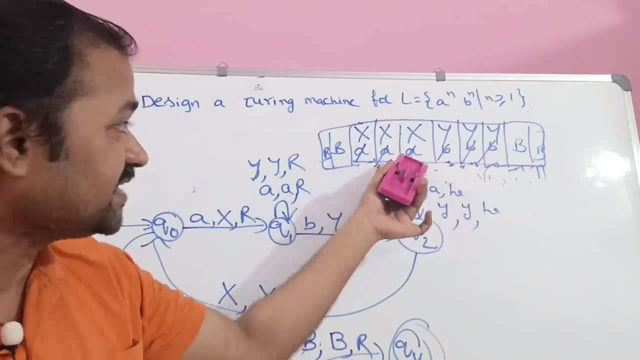 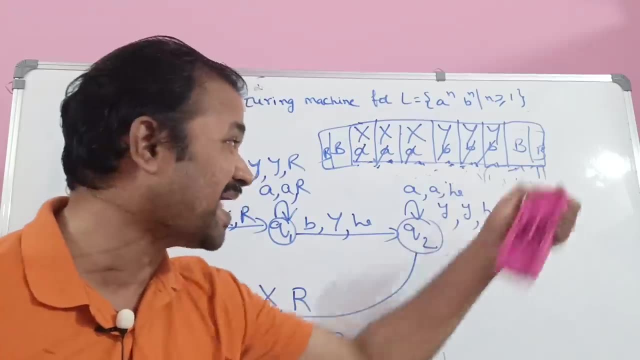 are replaced with x. we have 3 a's, So those are replaced with x's, and we have 3 b's. those are replaced with y, y, y, y, y, y, And after that we have got the blank spaces.